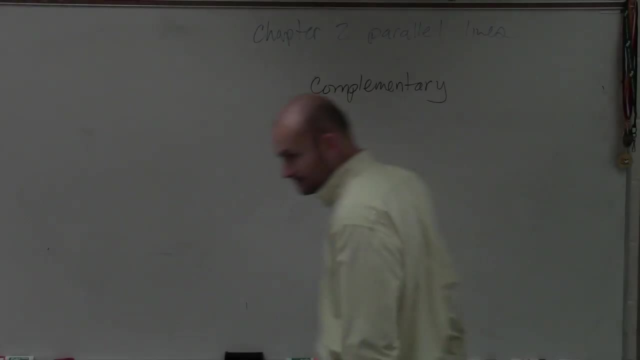 So, ladies and gentlemen, complementary angles- I'll just write out the formal definition and I'll show you what these are. Complementary are when the sum of two angles, when the sum of the sorry measure of two angles, is 180 degrees. Now, what am I doing? That's 90 degrees. 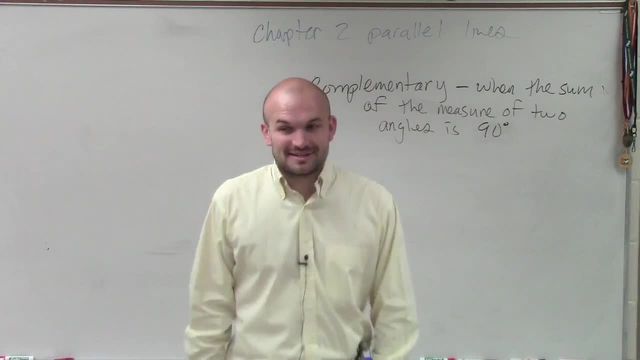 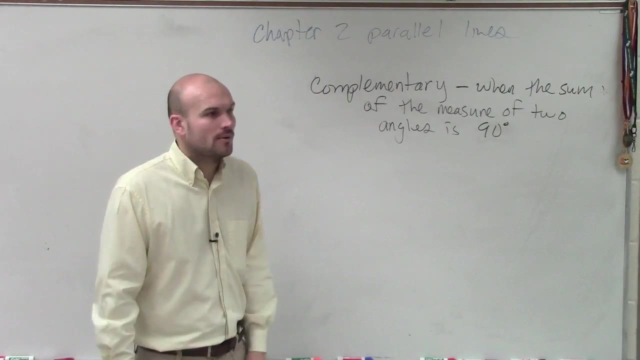 Sorry, I don't know if I was thinking about the next one or what, But yeah, it's 90 degrees. Sorry, sorry, sorry, sorry, 90 degrees, All right. So when do we know that the sum of the sorry measure of two angles is 180 degrees? 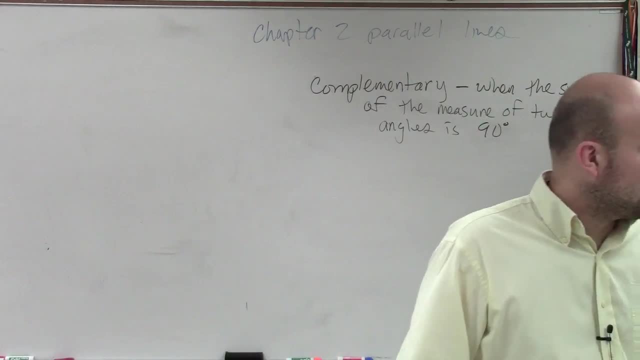 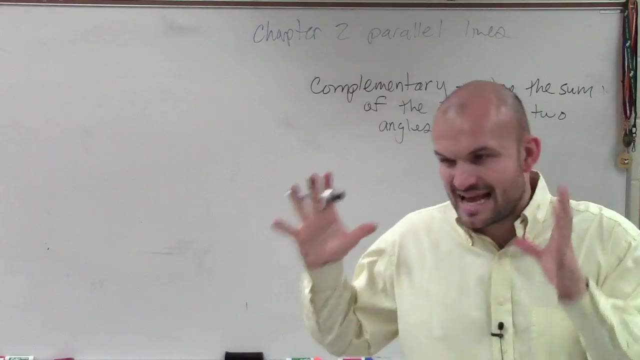 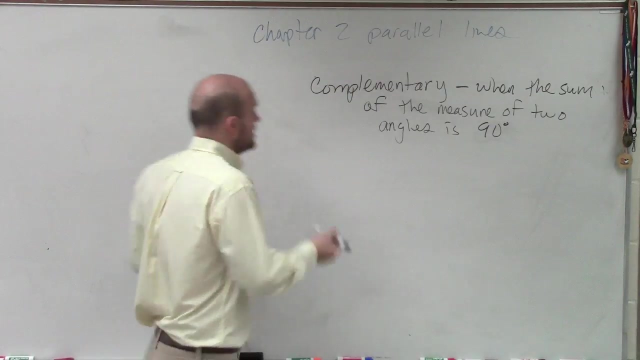 What do we know creates a 90 degree angle? Yes, 245s, yes, But what we've talked about in terms of angles, there's something on a picture that we used, yes, A right angle, And how do we know it's a right angle? That box, right. So what I just want to show you. 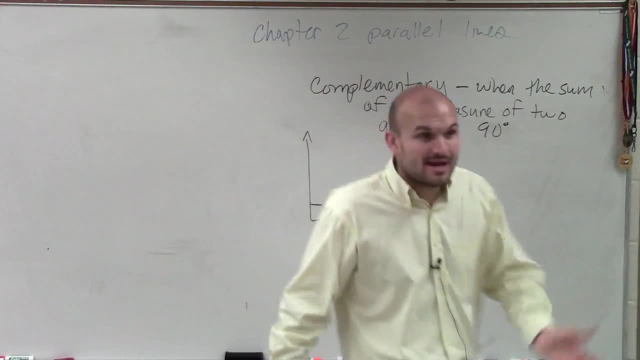 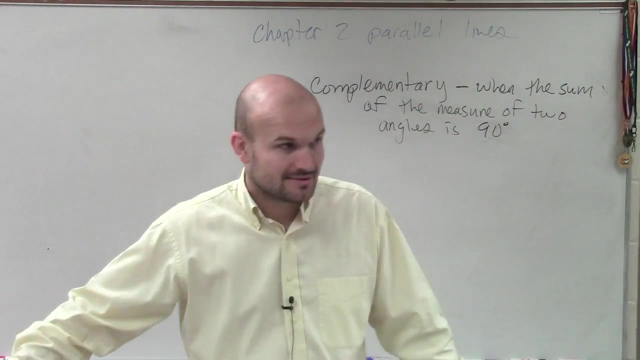 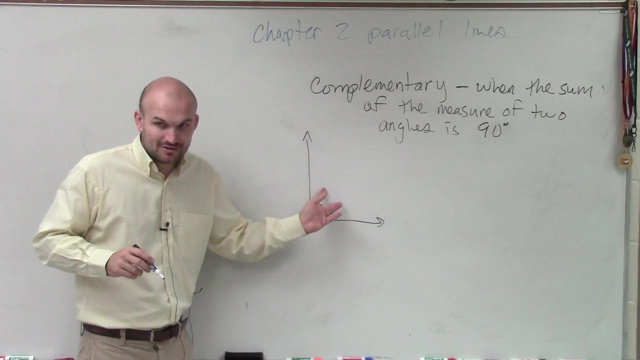 is that is a box right, That means it's a right angle, That means the degree measure of this angle is what? 90 degrees, Yes, Yes. So therefore, ladies and gentlemen, if I cut this angle at all into two angles, 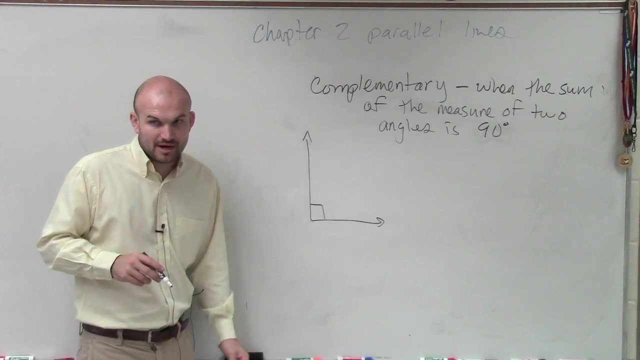 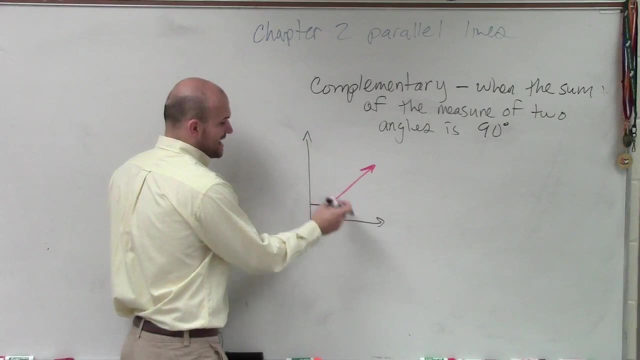 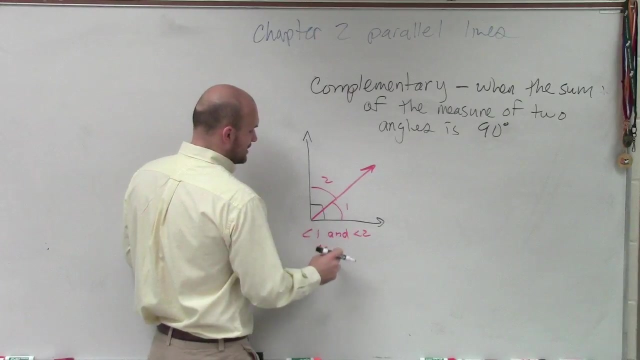 then we know that those two angles are going to be complementary, right? So if I say, let's say I draw a line like this right Now, I just broke this down into two angles, one and two. Well, guess what? Angle one and angle two are complementary. 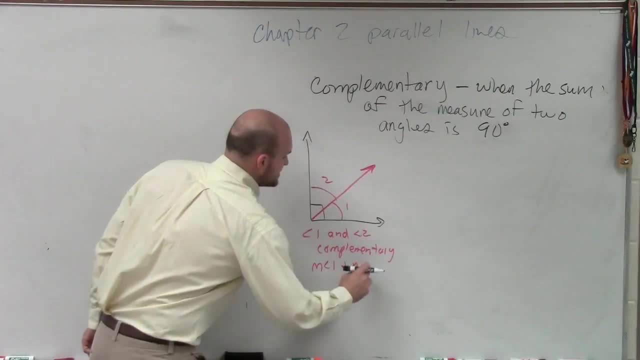 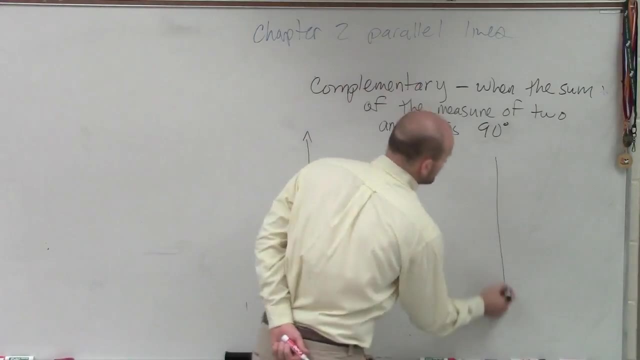 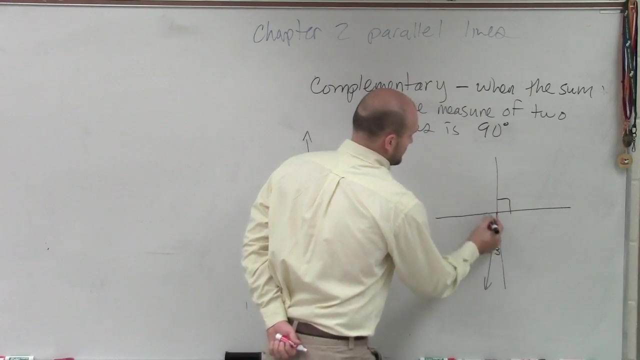 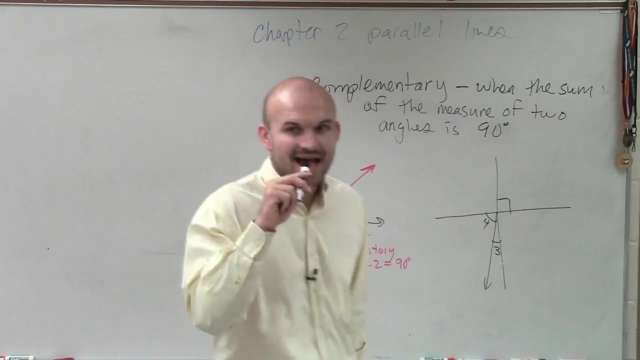 Right, Because the measure of angle one plus the measure of angle two equals 90 degrees. Does that make sense? All right, let's look at another example. Ooh, that's a good one, Mr McLogan, Are angles three and four complementary angles? I want to go to you, but I want to. 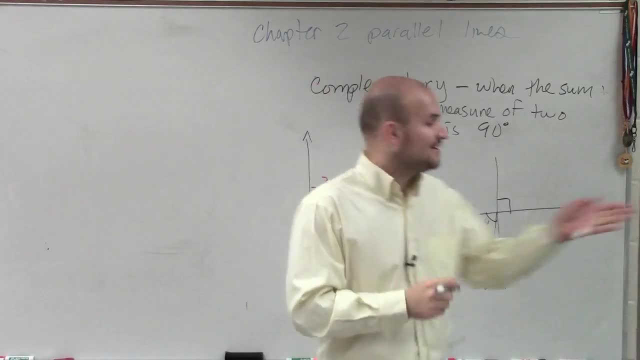 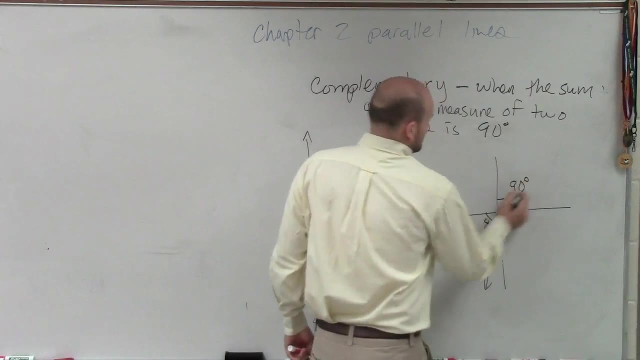 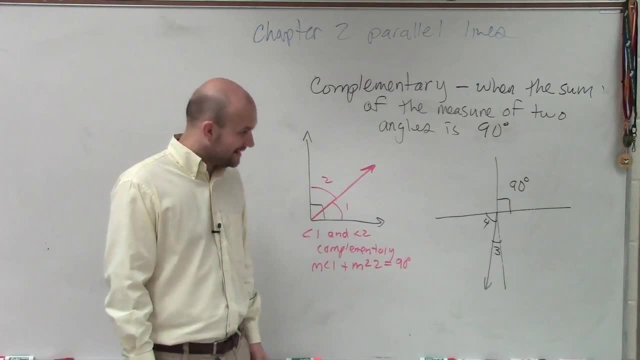 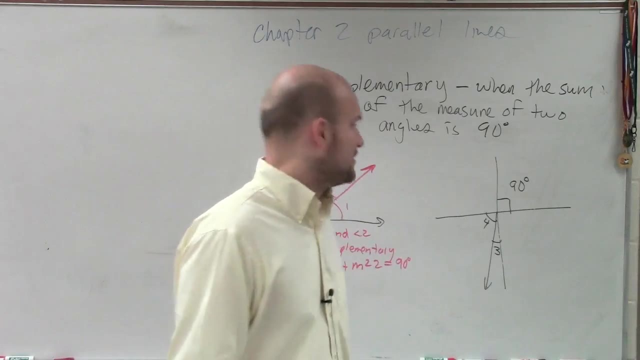 90. How do you know that? 80. It is the same, but how do you know they're the same? No, No, no, no. there's a definition that we talked about. What kind of angles are those? 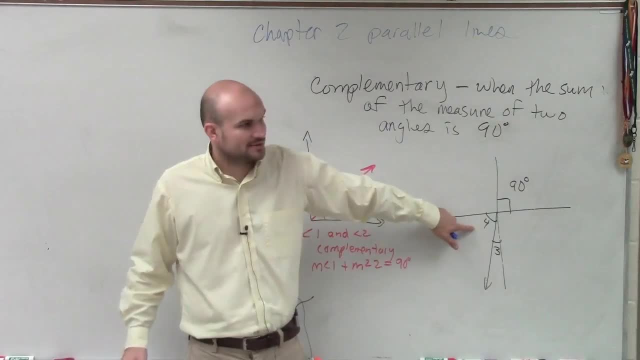 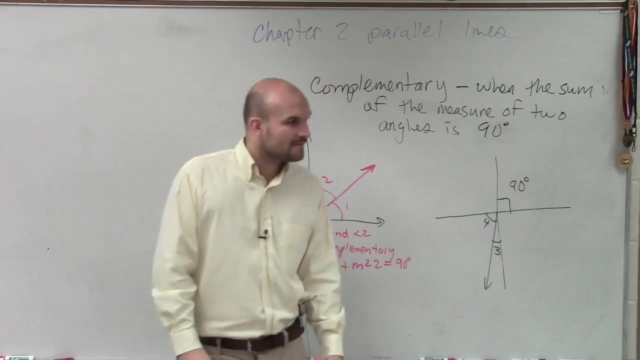 That is a right angle, You're right, but how is this angle, compared to this angle, Not close? I'm hearing a couple: You have adjacent or vertical. Which one do you want to choose? Make the right decision. Adjacent, So adjacent if we. 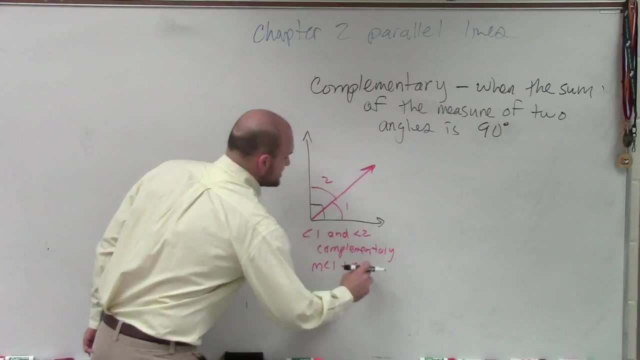 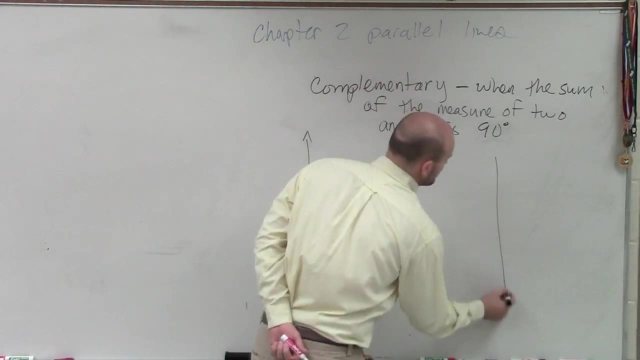 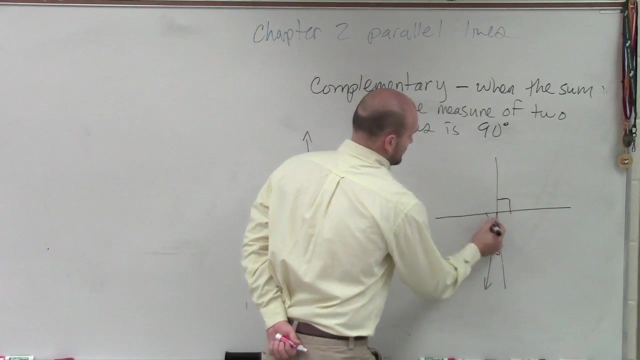 Right, Because the measure of angle one plus the measure of angle two equals 90 degrees. Does that make sense? All right, let's look at another example. Ooh, that's a good one, Mr McLogan. Are angles three and four complementary angles? 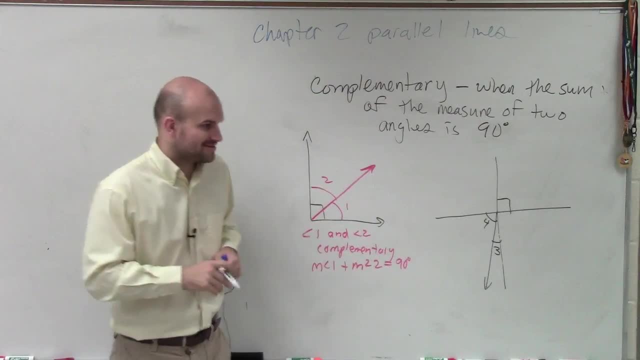 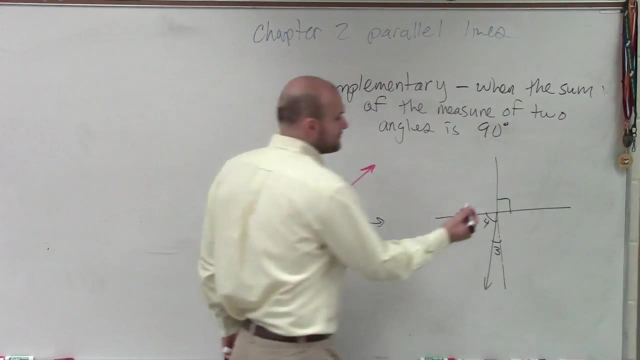 I want to go to you, but I want to try get some answers. No, No, No, No, No. What is this angle? What is the measure of this angle? 90. 90. Very good, What is the measure of this angle? 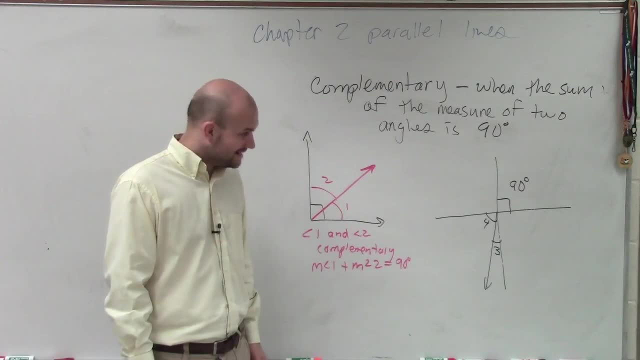 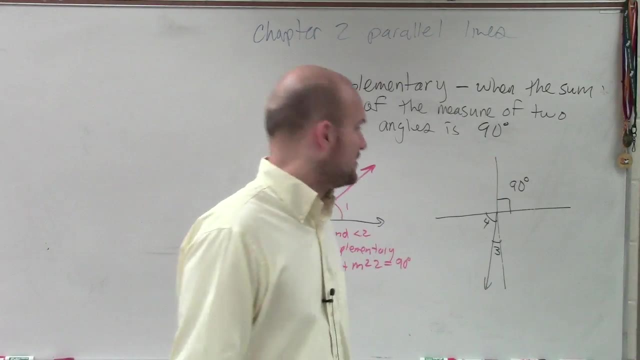 90. How do you know that It is the same? but how do you know they're the same? No, No, no, no, There's a definition that we talked about. What kind of angles are those? Right, That is a right angle, You're right, But how is this angle compared to this angle? 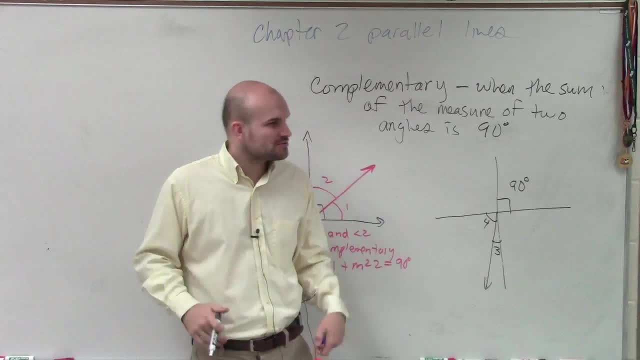 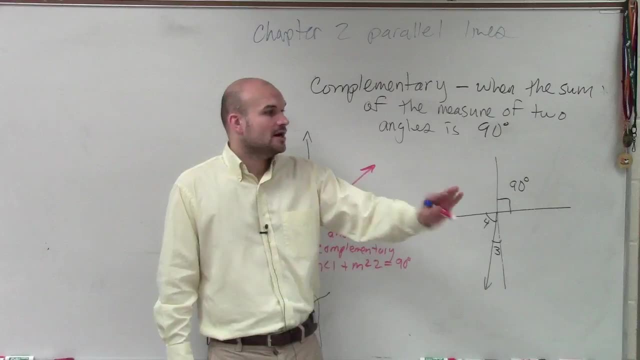 Not close. I'm hearing a couple. You have adjacent or vertical. Which one do you want to choose? Make the right decision. Adjacent, So adjacent. if we go back to our definition of adjacent, adjacent says they share the same vertex. Do those share the same vertex? Yes, 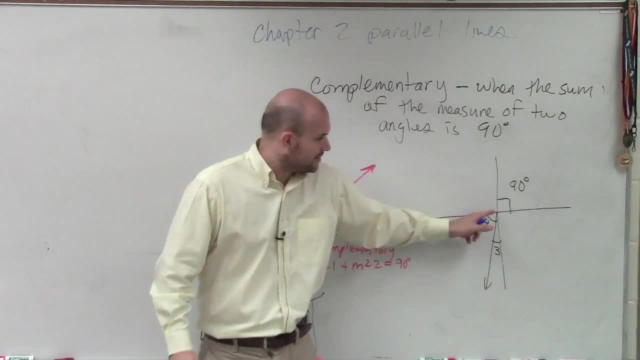 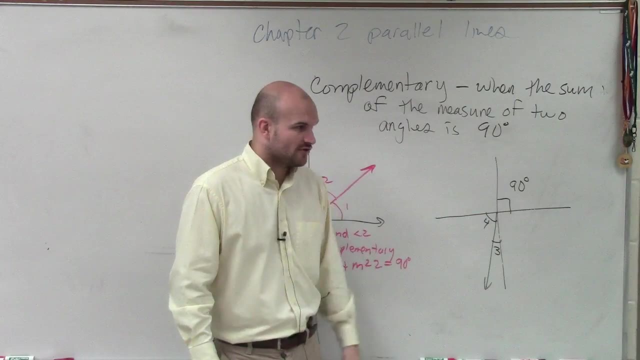 Adjacent says they share the same vertex and they share the same side. Does this angle and that angle share the same side? No, No, So they can't be adjacent. Let's go back to the definition of vertical Vertical angles. Vertical angles are one created by two intersecting lines. 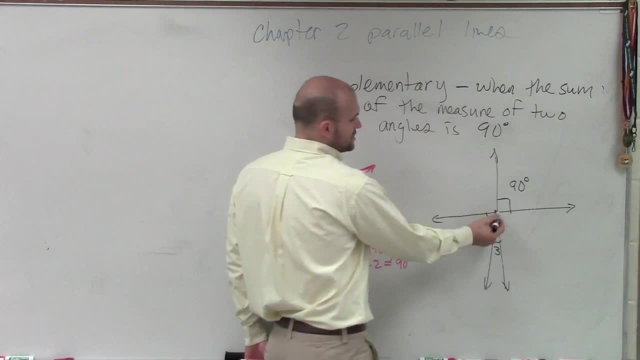 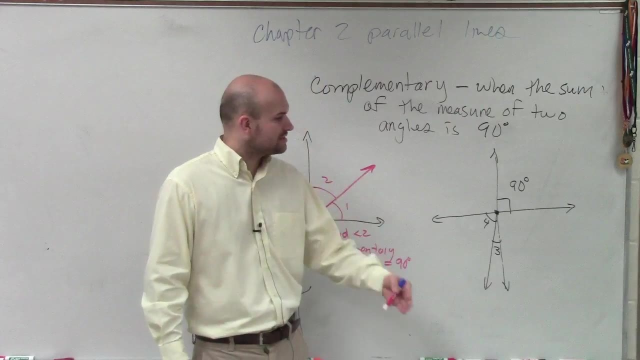 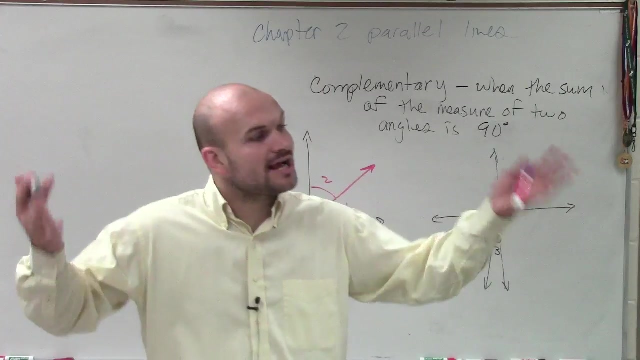 Are these created by two intersecting lines? Intersecting lines: Yes. Do they share the same end point? or vertex? Yes. Vertical angles also do not have any sides in common. Do these have any sides in common? No, So guess what? They're not adjacent, but they are vertical angles. 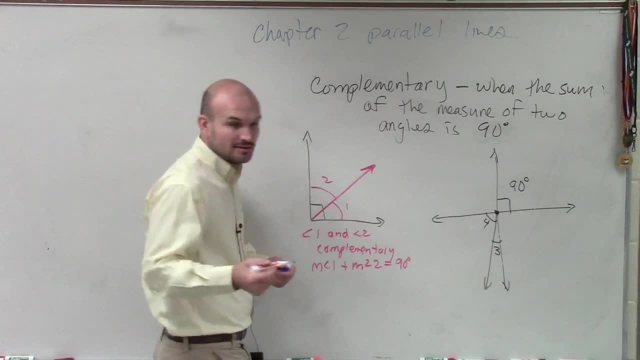 So, therefore, if this is 90 degrees, how many degrees is this 90.? So, therefore, is angle 3 plus angle 4 equal to 90?? Yes, Is angle 3 and angle 4 equal to 90? Yes. 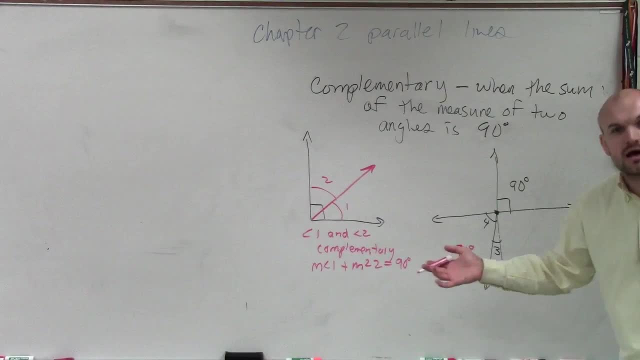 So these aren't vertical angles or, I'm sorry, complementary angles. Yes, they are. So you've got to say that angle 1 and angle 3,, I'm sorry, angle 4 and angle 3 are complementary. Okay.